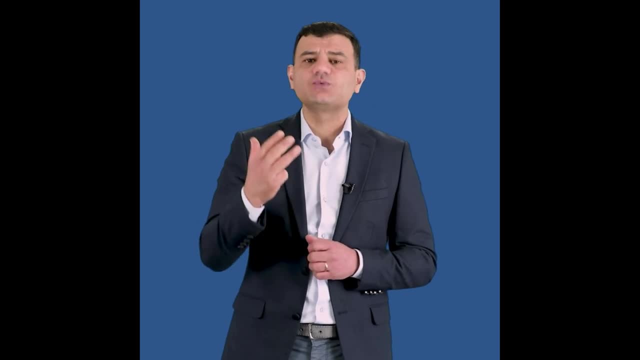 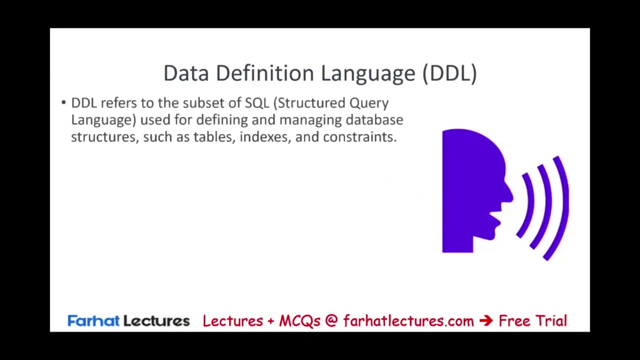 lectures, multiple choice questions, true-false questions, as well as exercises. Go ahead, start your free trial today. Data Definition Language, or DDL, is a subset of the SQL and it's used for what? Look at the term definition, used for defining and managing database structure such as tables. 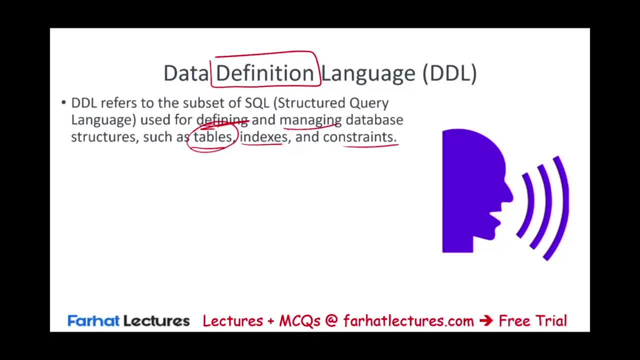 indexes and constraints, And we focus more on tables, but we will also discuss constraints as well. It helps build and modify the structure of the SQL. So let's get started. Let's get started The structure of a table. I hope you know what a table is. A database, a big database, could have. 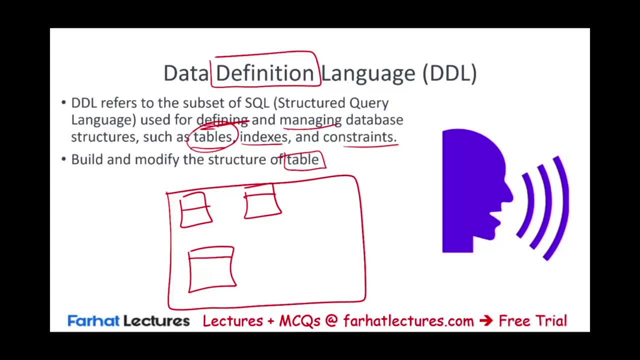 many, many different tables- Customer table, product table, order table, so on and so forth- And those tables are connected in one way or another, whether it's a one-to-one, one-to-many, many-to-many, so on and so forth. The assumption here is you know basic concepts about foreign. 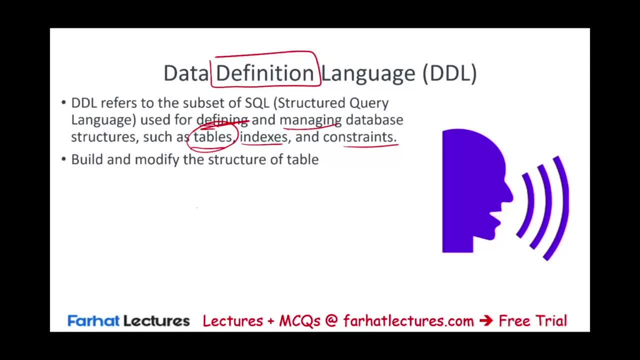 key, primary key relational database, But specifically the command we're going to be learning under the definition of the SQL. So let's get started, Let's get started, Let's get started. The data definition language are the create, the alter command, the drop command, the truncate. 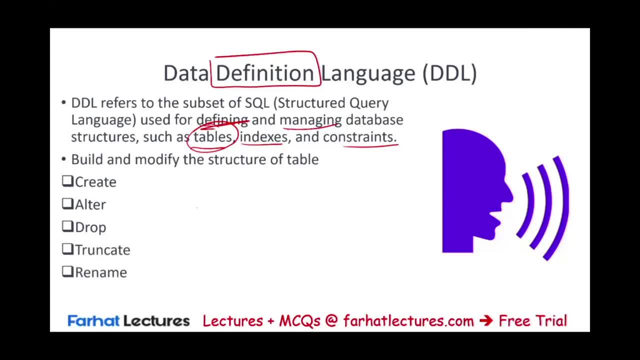 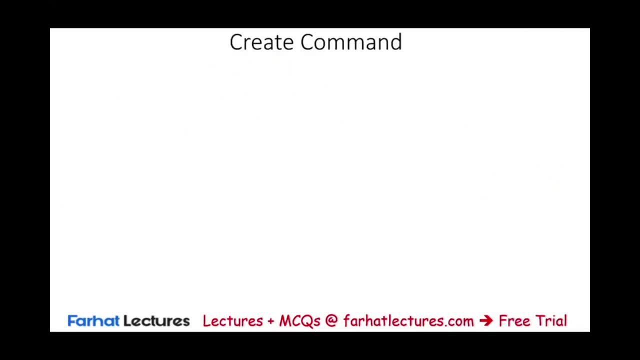 command and the rename command. In this lecture, I will focus on the create and alter command. Let's go ahead and start to discuss the create command. Well, as the word suggests, create command, What are we creating here? The create command is a foundational aspect of the database. 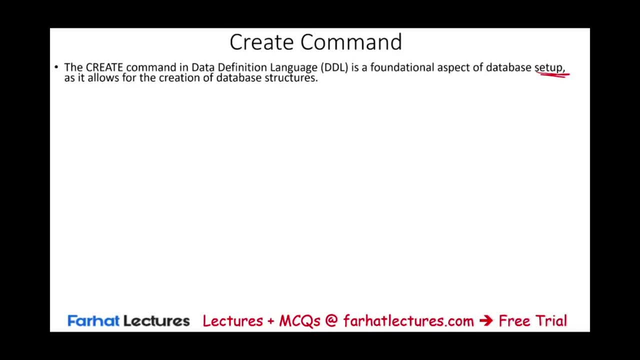 setup. We're setting up the database. The database is made of tables. So what are we creating? We are creating new tables and objects in the tables, So it allows the creation of database structure which is made of tables, While the create can be used for various objects, like 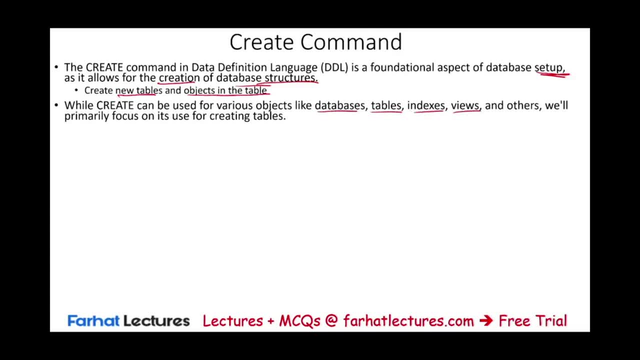 databases, tables, indexes, views. we will focus on the create command. We'll focus on tables, So this is our focus here: The create table statement. this is the order, the syntax, the programming. create table is used to define a new table, So we're focusing on 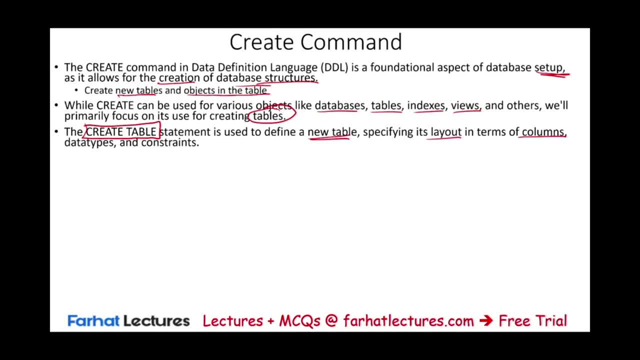 a new table specifying its layout in terms of columns, data type and constraint. So a table will have certain columns, layout, constraint, data type, something like this, For example: this is the language to create a table. We'll have the table name: column. 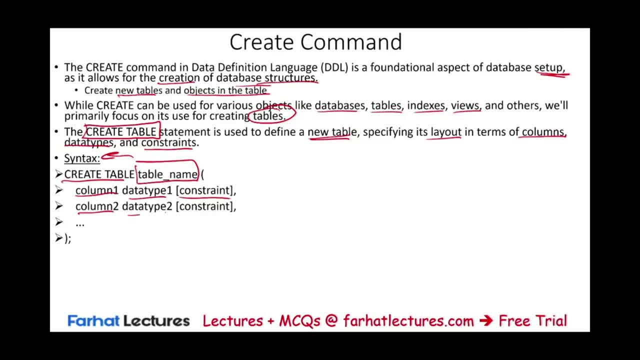 one data type. what's the constraint for the data Column? two data type. what's the constraint for the table? Specifically, let's take a look at a student table. So this table is a student table. That's the table name. 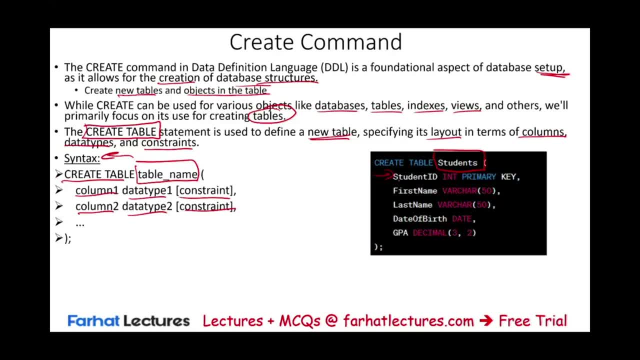 We are creating this table. The first column is student ID. It's made of integers. Integers is one, zero, one, two, three numbers. It's a primary key. So the student ID is the primary key. Then we have column two. We're going to add the first name of the individual. 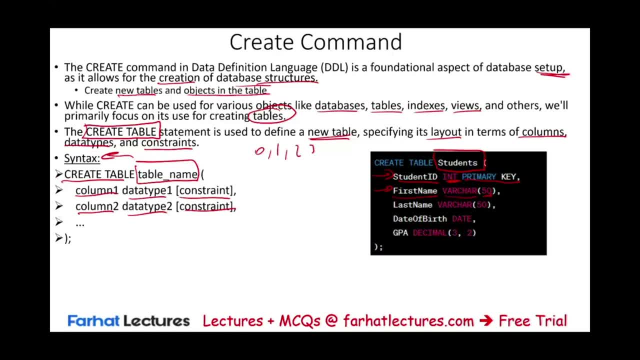 and this is going to be a variable character, up to 50 characters. Last name, also variable character. The date of birth will be a date, The GPA of that student, because we're dealing with a student decimal. You could have three numbers. Two of them are decimals. This is basically the way the 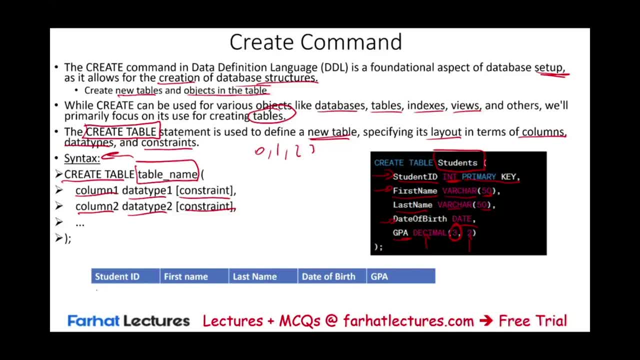 language is presented And this is what the table look like: Student ID. So we'll have the student ID- zero, zero, zero one- The name, last name, date of birth and GPA, And we'll have the record of many, many students. But this is the table. So the first thing, 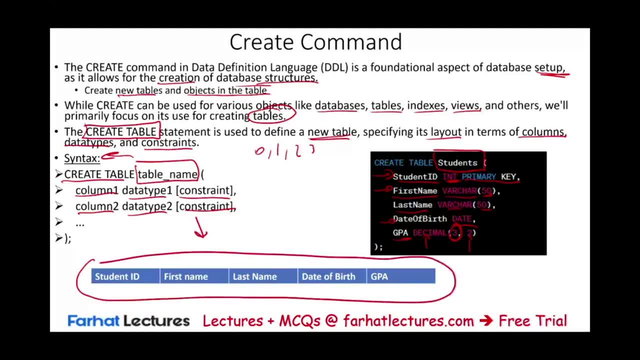 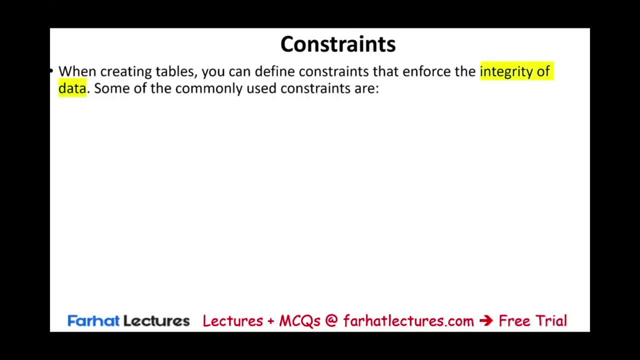 the create command will create the table, And this is what we did: We created a table, the create command. Now let's talk about the constraints. When creating a table, we're going to define the constraints that enforce the integrity of the data, And I hope you. 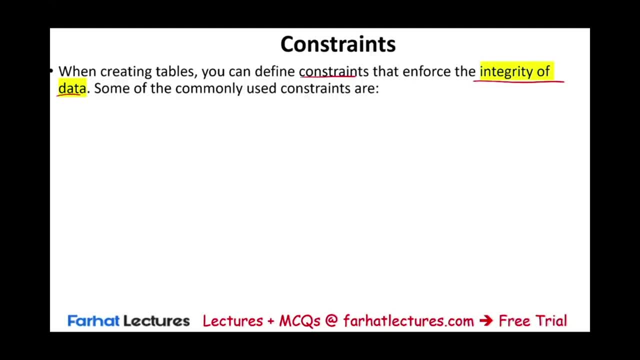 know about the integrity of the data. We have one whole session. It's part of the control of securing the database, making sure that the input that we are inputting has integrity. Some of the commonly used constraints are the primary key. What's the primary key? The 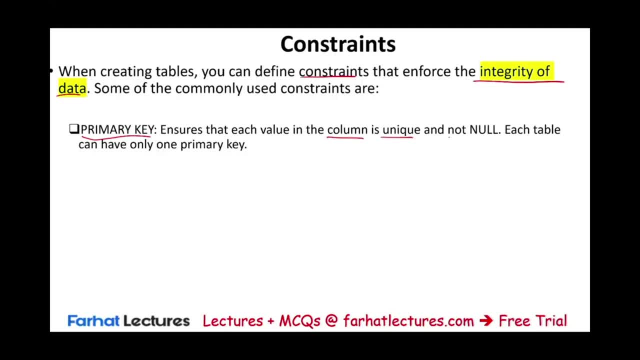 primary key ensures that each value in the column is unique and not null. Not null means we have to have something And each table will have one primary key that identifies uniquely that table. For example, in this example here, our primary key was the student. 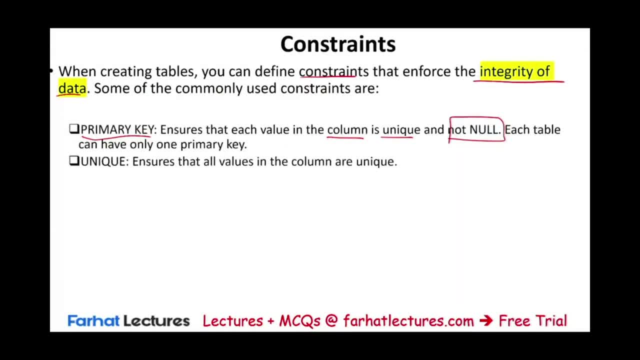 ID And I hope you know the difference between primary and foreign key. Unique: We want to ensure that all values in the column are unique. So the values in the column are unique. They're not the same as each other, Not null. We want to make sure that all columns cannot have 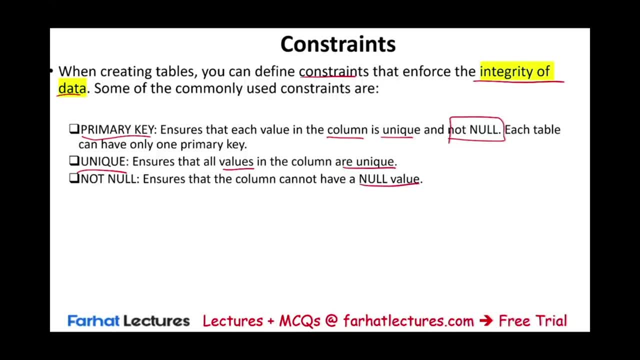 null value. You have to have something. Null means nothing. You have to have something. You want to have a foreign key. The foreign key is what establishes a link between the data and two tables. The foreign key is what creates the relationship where values in column must match values in some primary key in another. 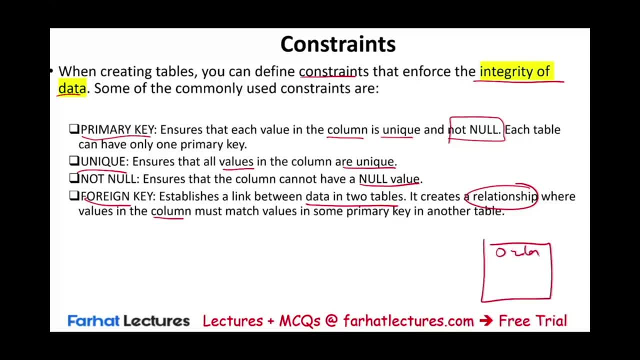 column, For example, we could have the order table And in the order table we would have the customer ID, the customer ID as the foreign key linking the customer to the order table. We would have check, which a check ensure that the value in the column satisfy a specified. 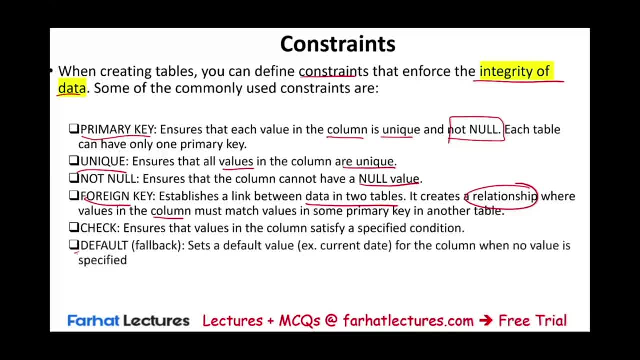 condition. We would look at it a short example, and also we would have a default, a default setup. a default setup is something that the column would default to if you did not enter anything. for example, if it's a date, if it's a field where you have to input the date and you don't put the date, it will automatically auto. 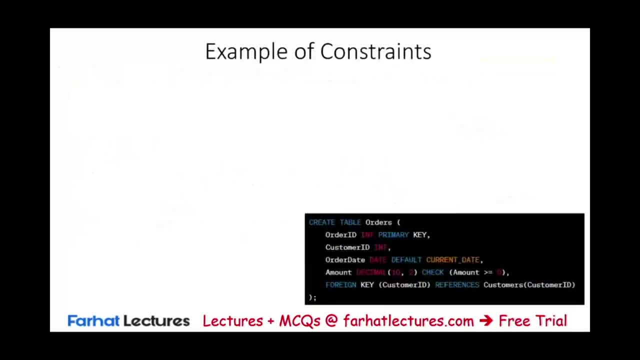 fill the current date. they basically it's a default. so let's take a look at an example of constraint. let's take a look at this table again. we have the order date, for example. the order date is the default. the default is the current date. so this is how, what the constraint is. so every 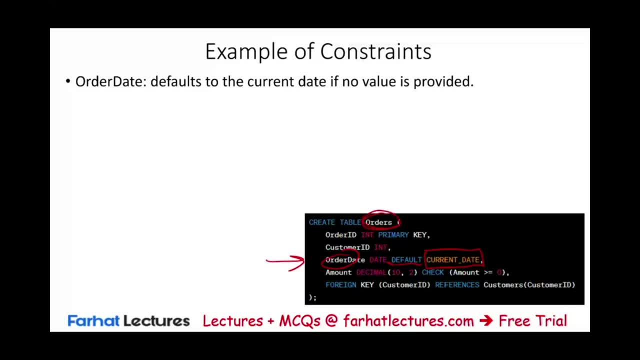 time you start a order tape, every time you start an order. this is order stable, not student order stable. we have an order ID. it's the primary key, the order date, the constraint it will automatically be there will have. amount must always be non-negative, so notice the amount it has to be. 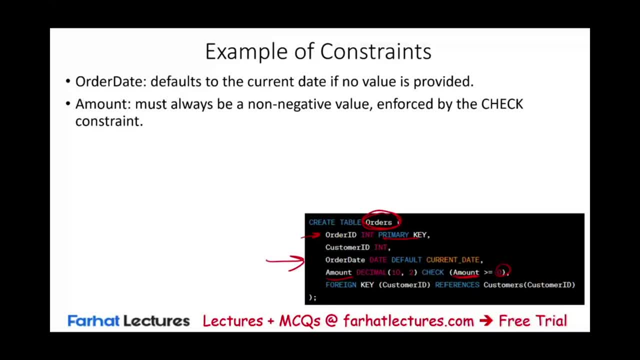 greater than or equal to zero, so the amount cannot be negative. we cannot have an order where we have to pay money. the amount has to be positive. we could have up to ten digits and two of them can be decimal. that's plenty of money for one order. 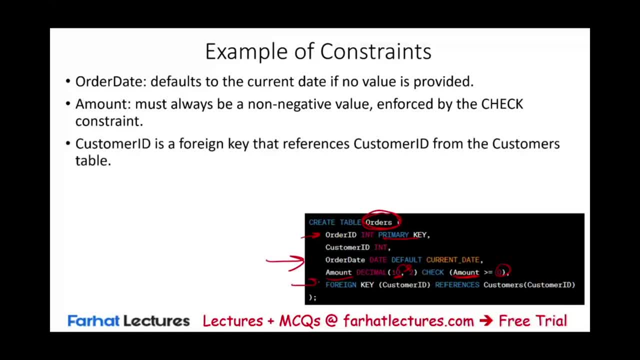 right. customer ID is the foreign key here. the customer ID must be included with the order because every order should have a customer. you cannot have an order without a customer. we should have a customer ID. this means that any value in the customer ID column of the order must. 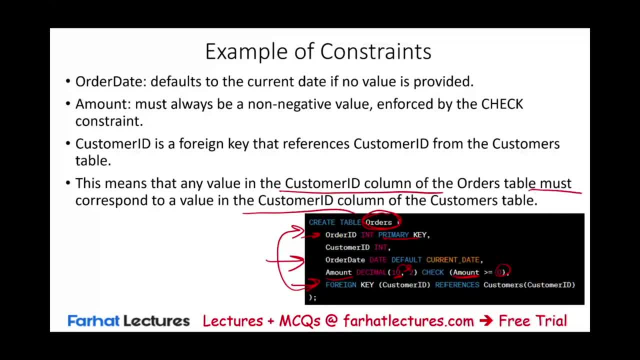 correspond to a value in the customer ID column of the customer table. so this is referencing we have. we have to reference some other customer. we cannot have an order without a customer. who are we selling the product to if we don't have a customer in the order table? and how do we link the customer? we link the customer through a foreign key. let's 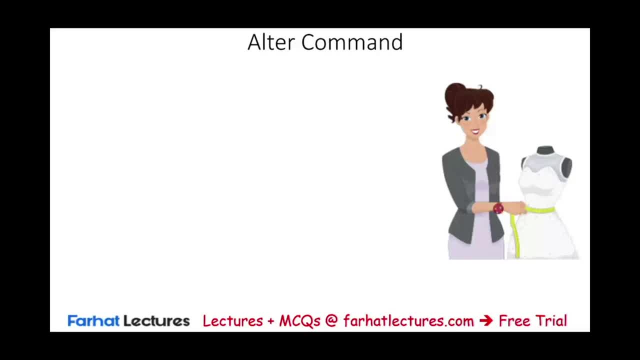 take a look now at the alter command: alteration, changing right. you're altering something different than create. we know what create is. create is create the tables and we showed you what we did. the alter command and SQL data definition data definition language is used to modify, alter, change, modify the structure of an existing database object, such as table we're altering. 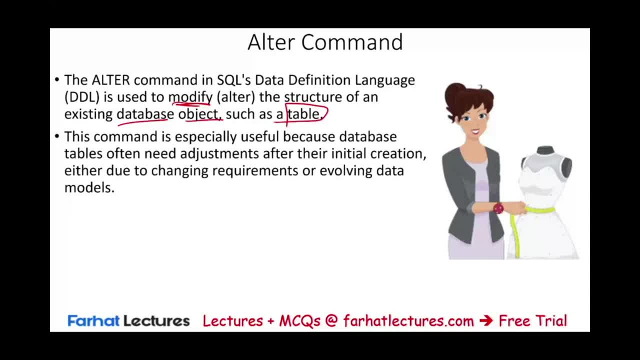 tables. here the command is specially useful. now, why do we have this alter? why do we alter the data? because over time we're gonna learn more about our business. we're gonna have new needs for the business, so we need to make adjustments. so the command is specially useful because database. 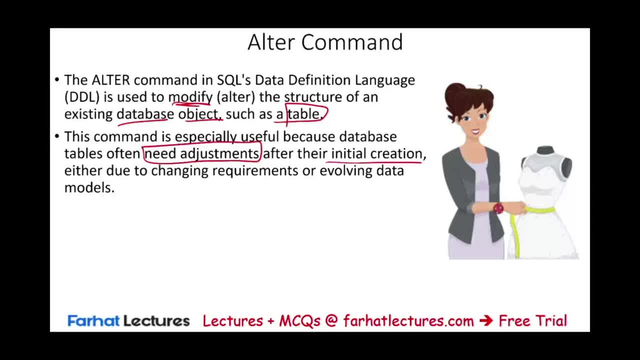 often need adjustments after their initial creation. this is what we think we need. then, once we started the business, we needed to change what we thought we need, either due to change in requirement or evolving data model. I'll give you an example, for example, let's assume we're only 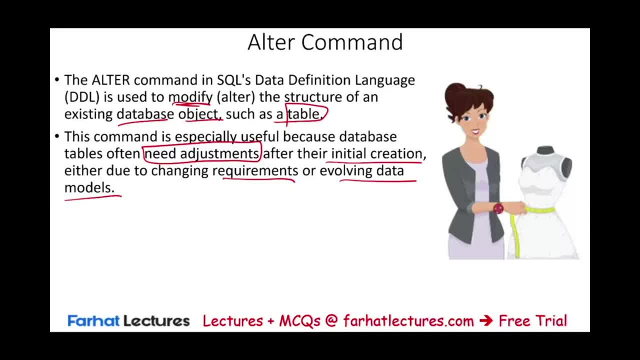 selling to us customers. so the address has to has a zip code. every address has to have a zip code. then suddenly we started to sell to international customers. well, some an internet internationally, they don't have a zip code. that's a five-digit zip code. so what we have to do, we have to go in and change the address constraints. so this is what we mean by. 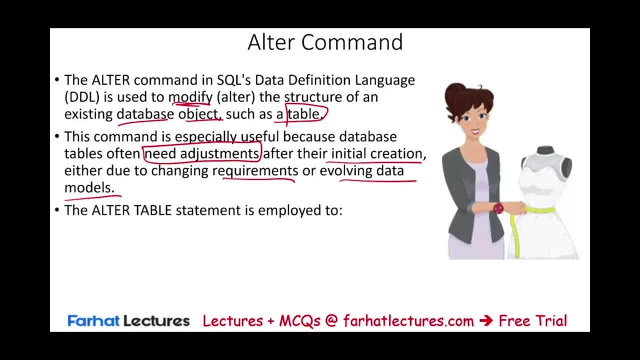 the need will change. so the alter table statement. so this is the command alter table statement- is employed to add, delete or modify columns. so we're looking. we're looking at the columns. we can add one, delete one or change the column, not the table. we're dealing with columns, columns or add, drop. 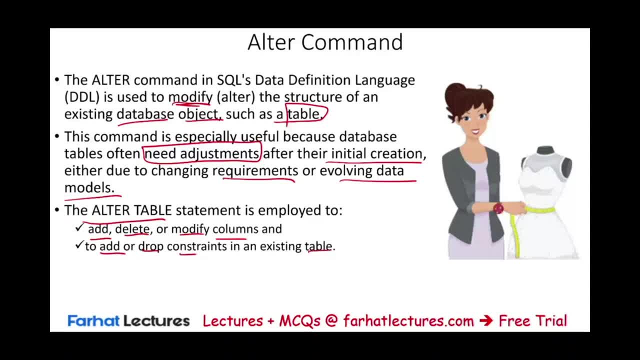 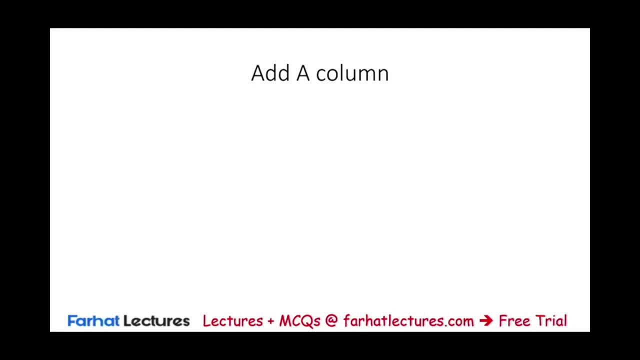 constraint an existing table or go to the constraint and change the constraint. whatever we need to change, let's start with add a column, just to kind of give you an idea what we are looking at. so the language would look something like this: alter table. that's the command. you put the table name. whatever the table name is. 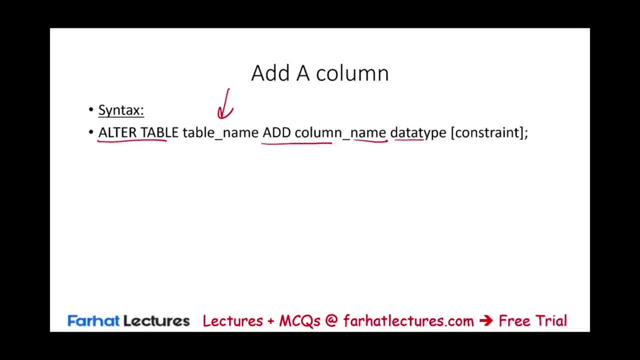 app column, name of the column, data type and what constraint you want to add. for example, alter table students- that's the table that we're altering- and add the email, and the email could be a variable character up to 100. in this case, we are adding a new column called email to the student table, so 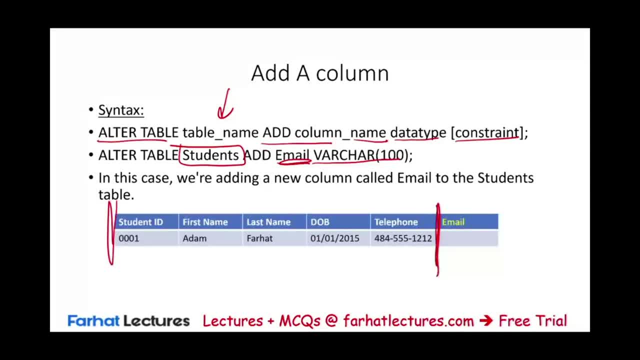 this is the student table. this is think of. this is the old student table. and now what we did? we added this email. so notice: what we did here is alter command. we did not go back and create a new table. we are altering an existing table. make sure you know the difference between create, basically when- 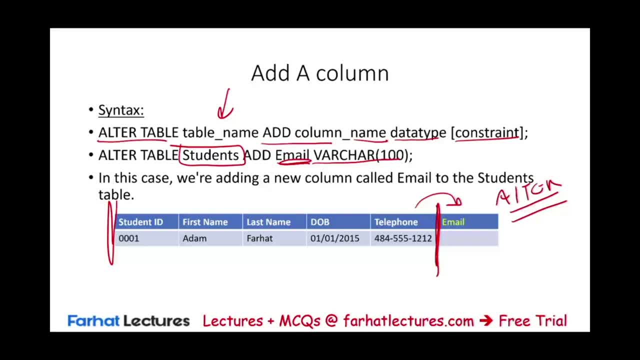 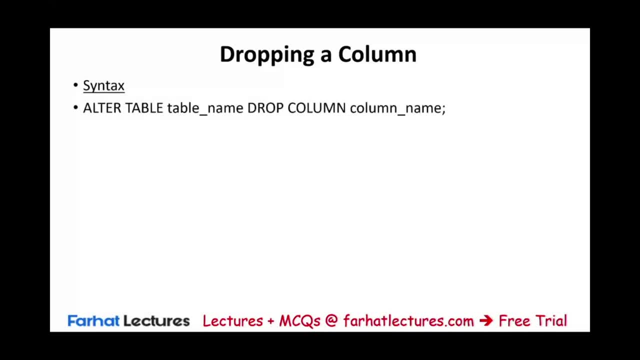 it's initially born, versus: you have the table and you're altering the table, just like we add a column. what can we do? you guessed it: we can drop a column. it would look something like this: alter, command the table name, whatever the table name, drop column is the order and you name the column. 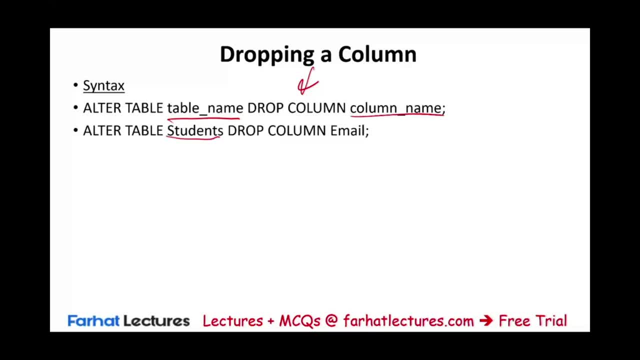 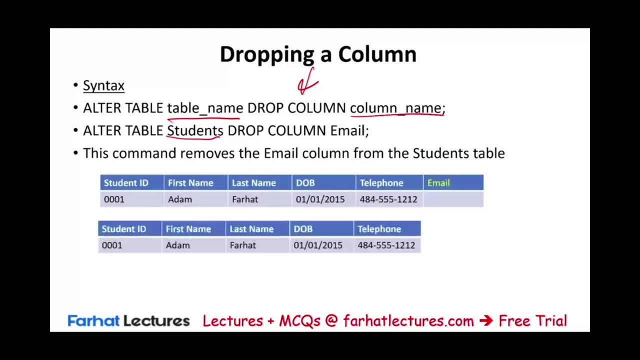 something like this: alter table, the student table, drop column email. well, the command removes the email column. so this is what it looked like earlier. now the email is gone and now we have this table. we alter the table so we can add the column, remove the column. now remember why am i? 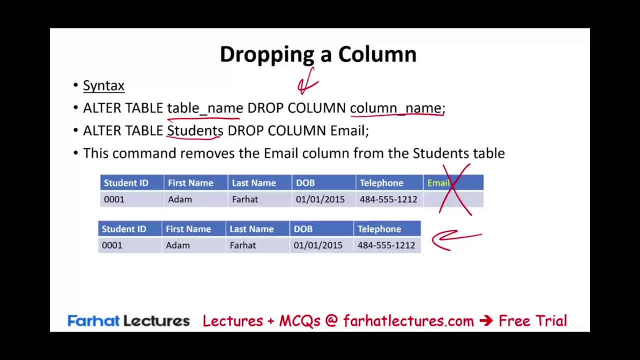 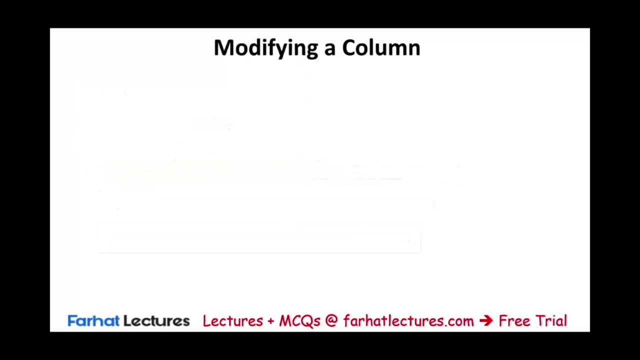 why am i mentioning this? because a drop in a column is totally different than dropping a table different. so make sure we understand. we are working with columns here, not the whole table. we're not dealing with table, because that's a totally different command. when you drop a table, you could modify a column. what's modified, make some changes. this action is used to modify. 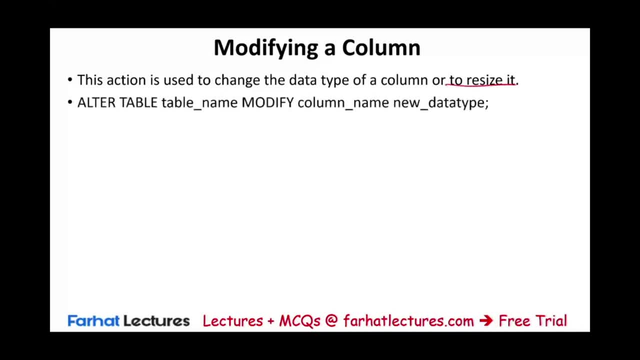 the data type of a column or to resize it. for example, alter table. you put the table name, modify column. whatever you want to do- new data type, for example, alter table. students modify first name rather than 50, make it 100. we're resizing it. some names: they need 100. 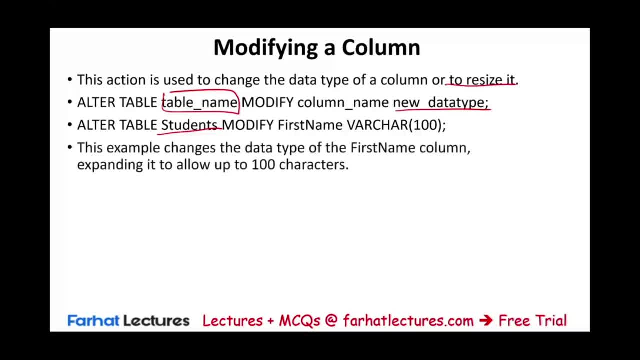 characters, so therefore make it better than 50. we have names that are one close to 100. this example changes the data type of the first name, expanded it to allow 100 up to 100 characters. for example, here we have adam. adam is four characters, but we could have 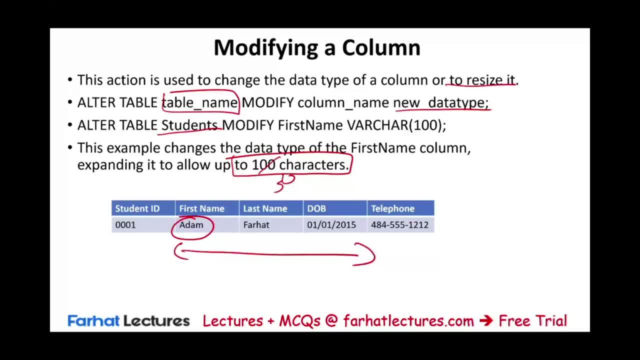 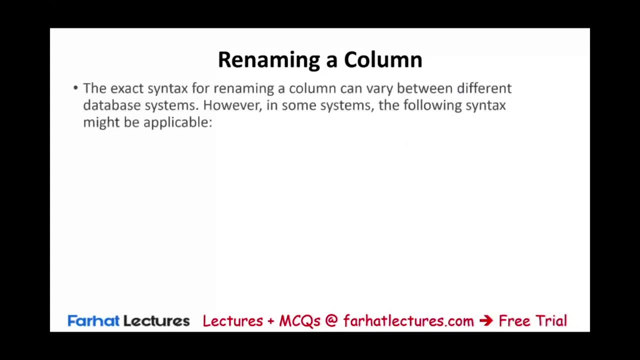 a name that's way larger. before it was 50, now we want to increase that because we find out that we have customers with more than 50 names, 50 characters in their first name. therefore, what do we do? we modify the column. we don't create a new table. we modify the existing column. we could rename a column. well, the exact. 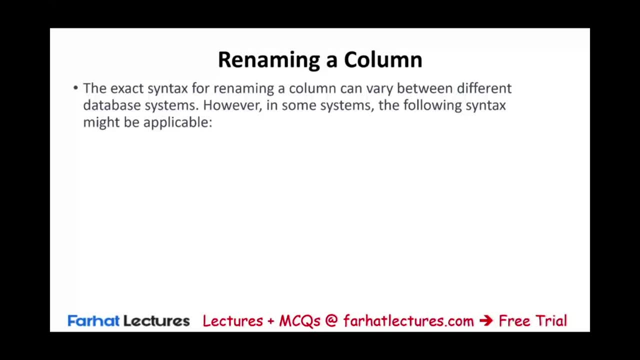 syntax for renaming a column can vary between database system. however, again we're using general sql. the following syntax will be used: alter table. we put the table name rename column- whatever the old column is name, to whatever you want to name the new column, something like change the telephone. 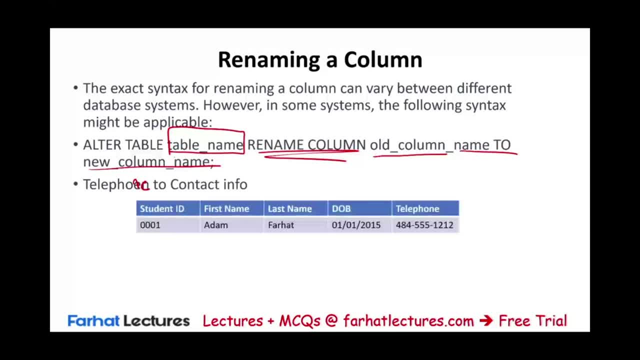 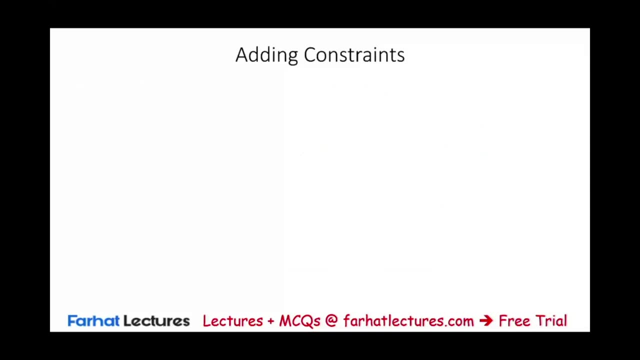 this is ne to contact information. so this is the old table where we have the telephone and we want to change that to contact info. we're renaming a column, that's fine, that's acceptable. what do we do we alter? we alter this adding constraints. you can also add constraint like primary key. 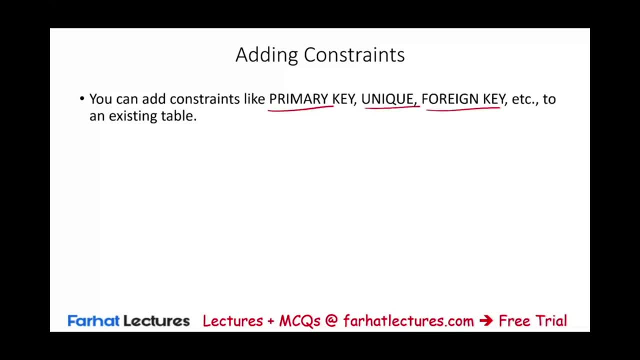 unique key, foreign key, etc. so an existing table. obviously you could have only one primary key, but you may want to alter that one. alter table name, add constraint. constraint indexes the programming: we're not concerned about the programming, I'm just showing it to you. so just to allow change, the simple. 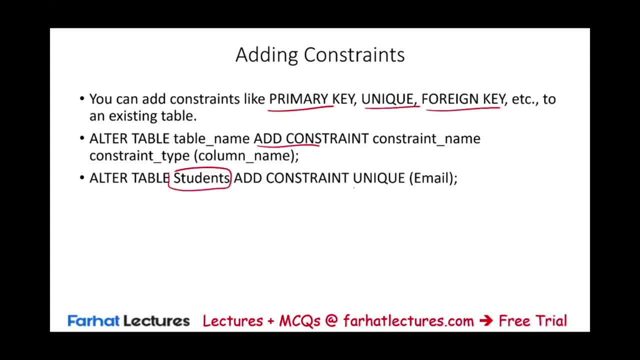 example, alter table student at constrained unique email. so every customer should have a unique email to ensure that email column and the student has unique values. so no one student can have to the same email. basically we're saying is, if this is an email, if you're putting an email, let's go back here to the table. I should have showed you the table here. 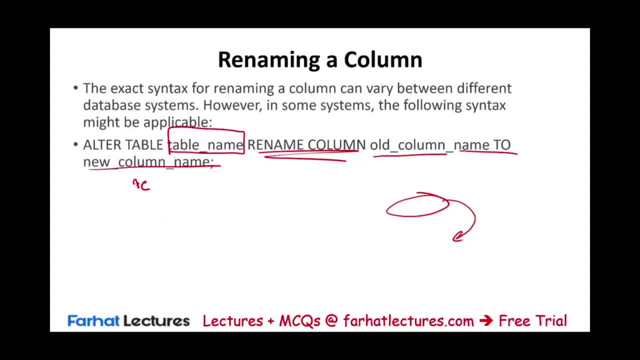 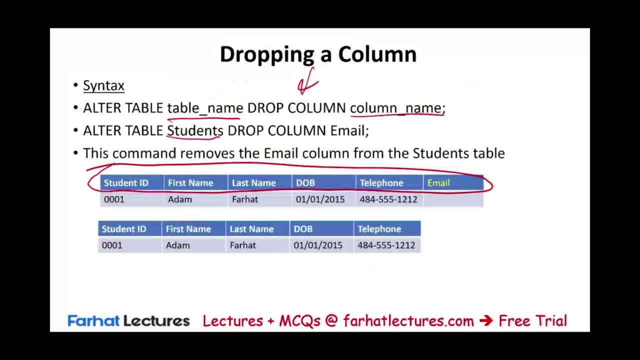 um, We don't have an email, but let's assume, go back to the table email. What we're saying here is: you cannot have a same student with the same email, So each email here has to be unique to one student. That's what we're saying. 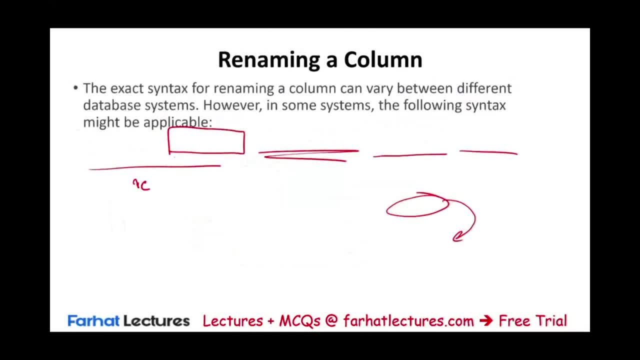 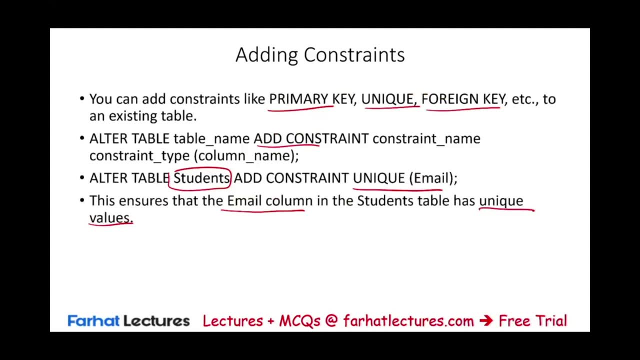 Unique. that column has to be unique. It cannot be the same. If you put someone's email, they'll say it will be rejected. It doesn't work because we added that constraint: that email has to be unique. In the email it has to be, for example, name at some serverorgcom. 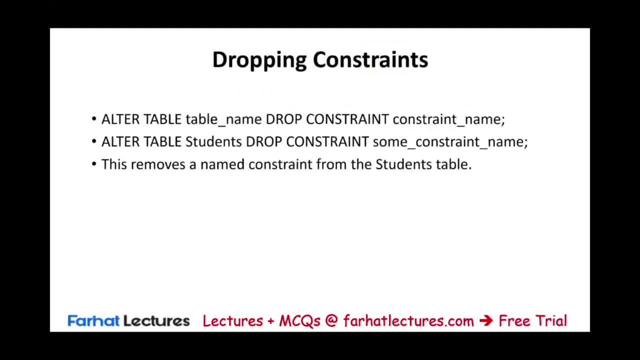 something like this as well: We can drop a constraint also. We can add a constraint. We can also drop a constraint. For example, alter table. whatever the table we're altering, drop a certain constraint. Alter table, student. drop constraint. some constraint name. 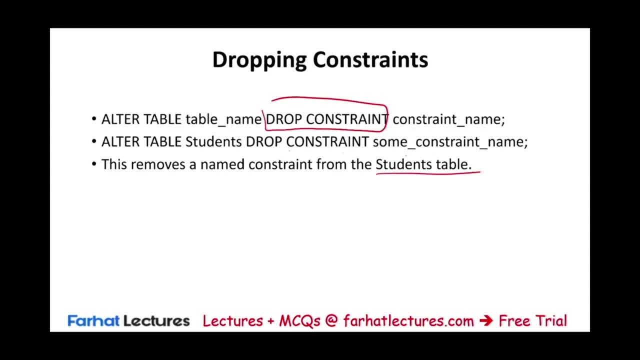 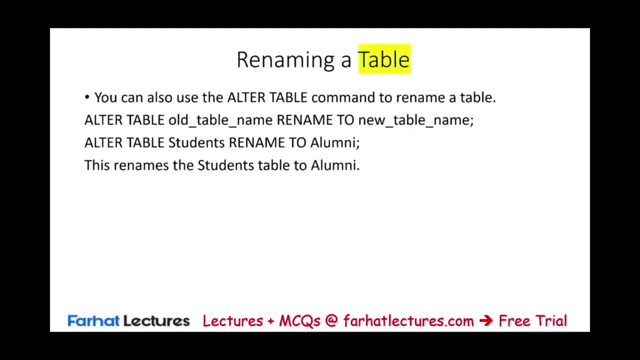 Whatever you want to do, just remove a name constraint. if we have a name constraint from the student table, For example, now we could use numbers or whatever we want to do in the name column. Renaming a table. Well, renaming a table. 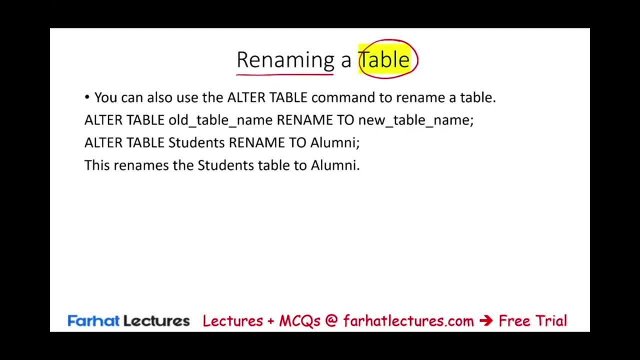 Notice: now we are dealing with a table. When you rename a table, you don't create a new table. It was already created under the create column. Renaming a table is under the alter command. So the reason I'm mentioning this. 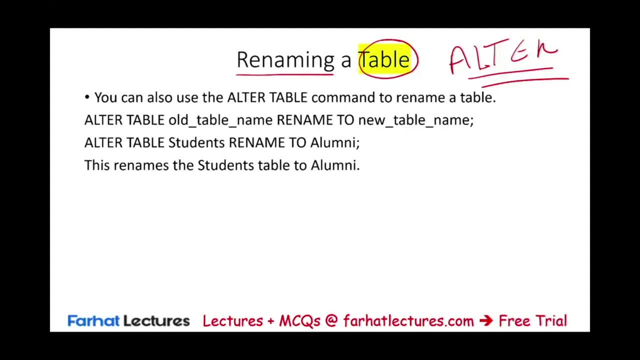 because this is what you're going to be tested about: knowing these commands. You could also alter table command to rename a table. You cannot drop a table, but you can rename a table. Okay. So for example, here what we want to do: alter table students rename to alumni. 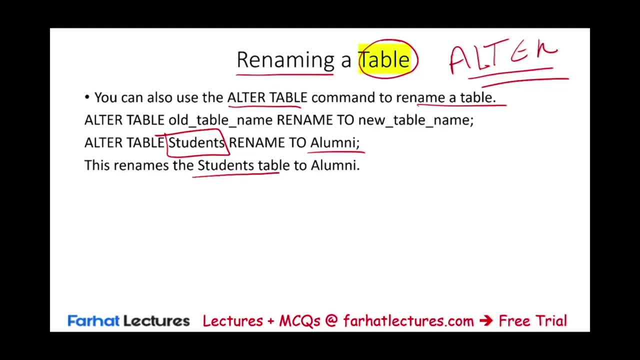 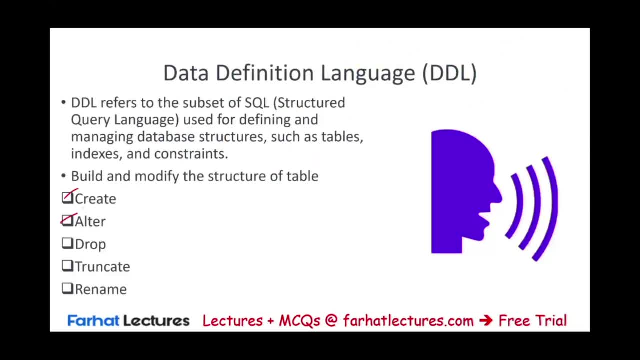 So we want to change the students table. We don't want to call it students, We want to call it alumni. now, That's fine. So what we did in this session is we looked at, create and alter, And the best way to kind of test our knowledge is to take a look at an example. 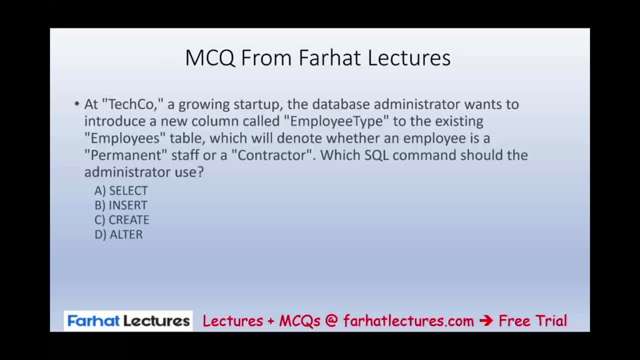 Let's take a look at this. multiple choice questions from Farhat lectures at Techco, The growing Startup. The database administrator wants to introduce a new column called employee type to the existing employee table, which will denote whether an employee is a permanent staff or. 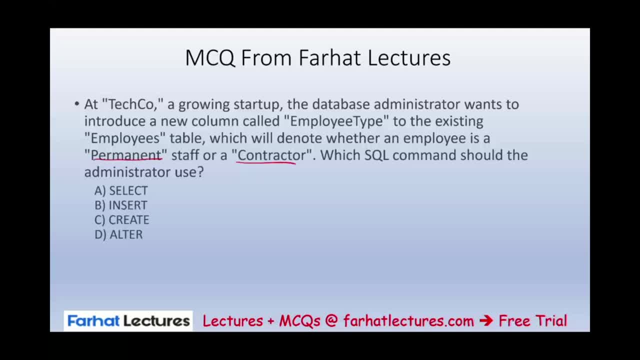 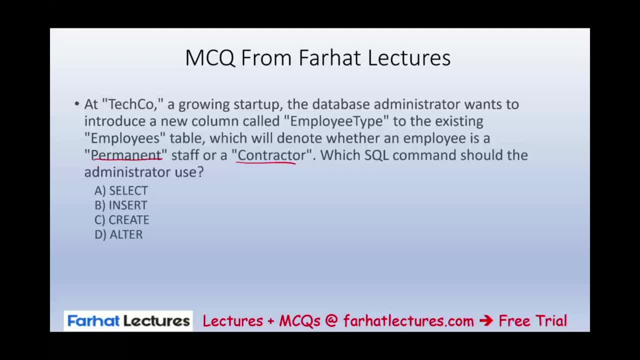 What does that mean? It means the answer must be: either, In this session we either covered create or alter. So what is the select? just to kind of to cover it real quick, We'll we'll explain it in different session- is used for retrieving data from a table, not for modifying its structure.